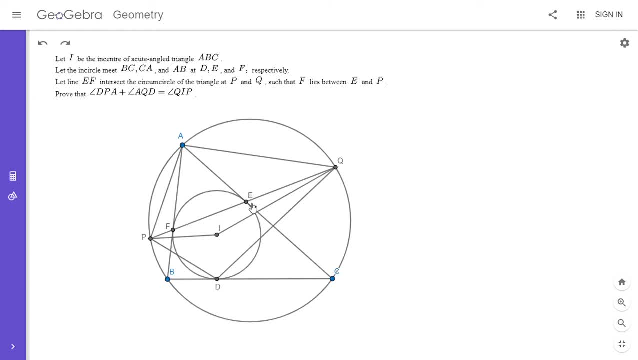 and AB, at DE and F, And then we draw the line EF and we let it hit the circum-circle at P and Q as shown, and then we want to prove that angle DPA plus angle AQD is equal to angle QIP, So not a. 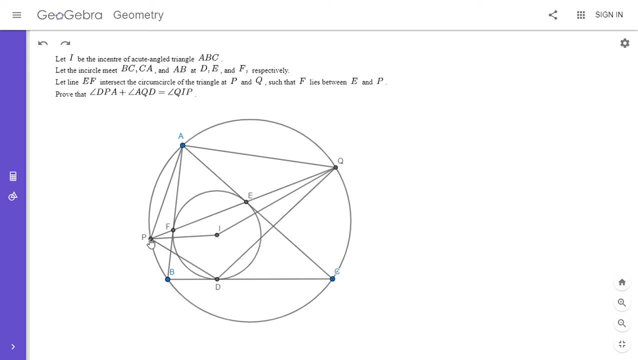 huge deal, but it is not a big deal, So let's get started. So if you have a complicated configuration but it's hard to kind of wrap your head around how to show the sort of angle sum condition, Alright. so one of the first things I 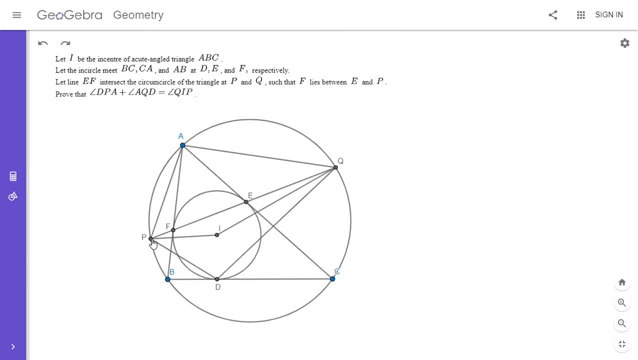 noticed, which I feel like really is a key to kicking off. the solution is that EF is the polar of A with respect to the in-circle. So, since AE and AF are both tangent to the in-circle, EF is the polar, So I mentioned that in video number 75. 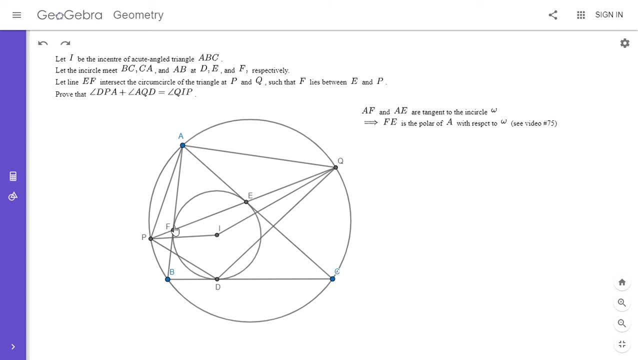 on my channel that the line joining the two points of tangency is the polar, okay, And so P and Q have to both lie on that polar, Alright, so if P lies on the polar of A, then that means that A has to lie on the polar of P. So basically, the polar of. 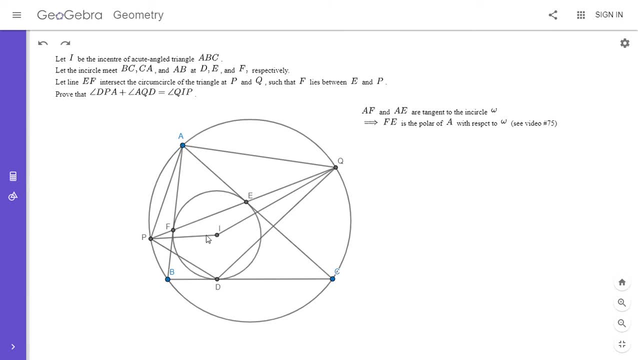 P. that's a line perpendicular to IP, And so what I'm going to do is I'm going to drop a perpendicular from A to IP. So this is what I mentioned: Since P lies on the polar of A, then A has to lie on the polar of P. That's Lahiri's theorem. so that's. 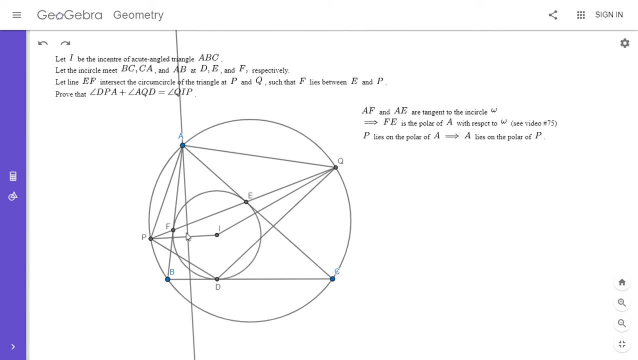 also in video 75.. So I'm dropping a perpendicular from A to PI and I'm going to let, I'm going to label three of the intersection points. So I'm going to label G, the intersection with EF, H, the intersection with IP, and J, the intersection. 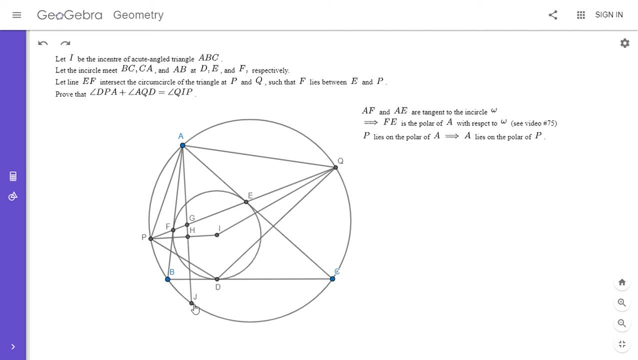 with the circumcircle, Alright, Okay, So where do we go from here? So G we labeled the intersection of this, this line, with EF. So G then also has to lie on the polar of, and so we can take advantage of that fact, because that means that we know that F, E, G and P are 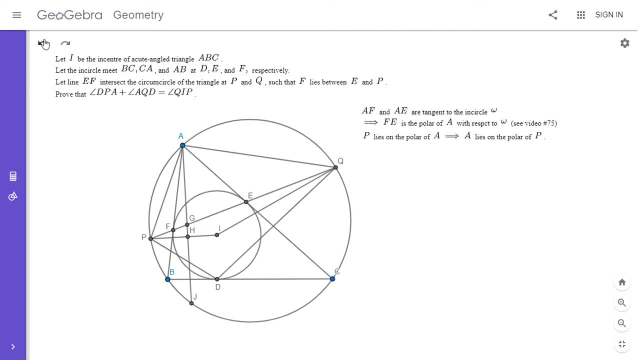 in harmonic conjugation. So this is actually from video 76 on my channel, so I'm going to write it out. So G, since it lies on EF, G is also on the polar P, and so the cross ratio F, E, G, P has to. 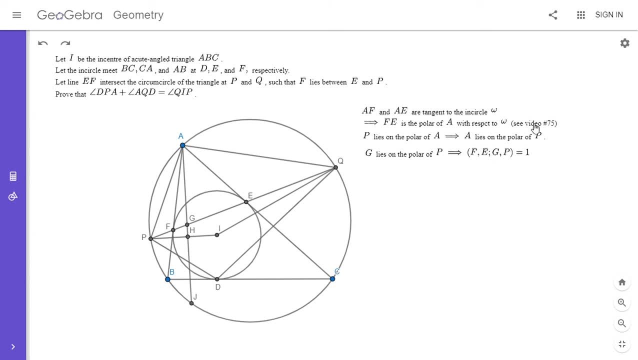 equal one. So this is the first theorem in video number 76 on my channel. I forgot to write it out here, but it's a super useful theorem, so I'd recommend checking out video 76 if you haven't seen this before. Okay, and once we have a cross ratio equal to one, then we can do lots of 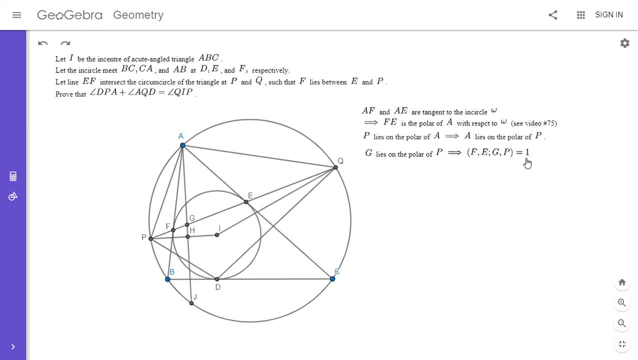 projections, and that often helps make a lot of progress. So we have F, E, G, P. What's a good point to project those four points through? So we can project point A through each of those four points onto the circumcircle, and so that's what I'm going to do here. So if we project those four, 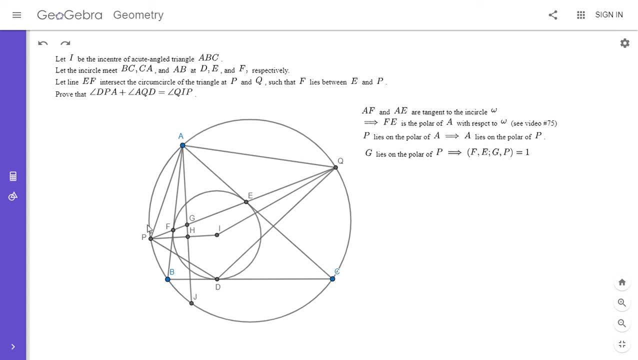 points through A onto the circumcircle. P stays at P, F goes to point B, G goes to point J and E goes to point C. So that's pretty convenient. so I'm going to write that out. All right, so we're projecting those four points through A, and so that's what I'm going to do here. So if we project, 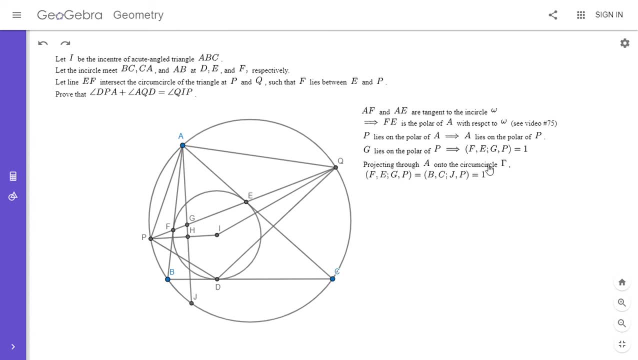 through A onto the circumcircle, which I've called gamma. so F goes to B, E goes to C, G goes to J and P stays at P, and it's still equal to one. All right, and we can do the same thing. So everything. 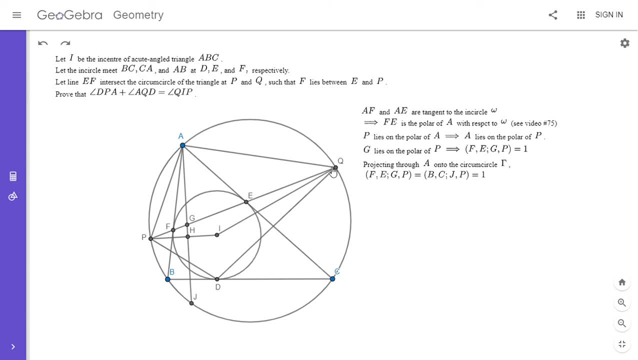 we've done. we've just done with respect to P, but we can do the exact same thing with respect to point Q. So I'm going to do that here. So I'm going to drop a perpendicular from A to QI and that has to be the point Q. So I'm going to do that here. So I'm going to drop a perpendicular. 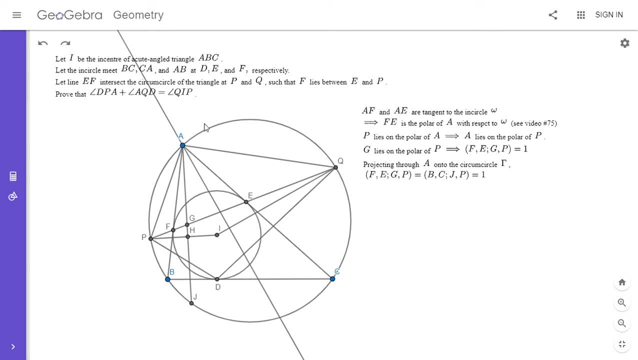 the polar of Q, from what I mentioned before. So now I'm going to label the intersection points KL and M, and we have to have the cross ratio: BCMQ is equal to one. Okay, so where do we go from here? We have the cross ratio: BCJP is equal to one. and we also have the cross ratio: BCMQ is equal to one. 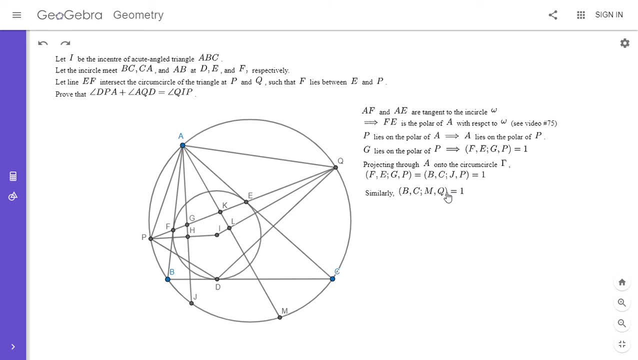 Well, just from seeing these two, I immediately had recognized- because I'd seen this before- that BC, PM and QJ all have to be concurrent. So I'm going to prove this out here for you, but I've done a very similar. 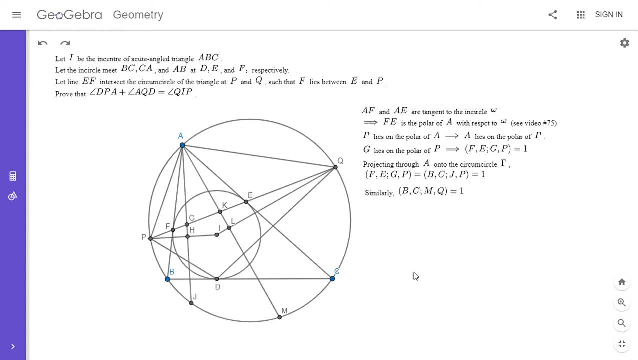 proof on my channel before. So if you look at my video on Pascal's theorem- I think it was probably around video 51 or so- and you look at the video before that, I do a very similar thing where I have two of these cross ratios equal to one, like this, and if two of the four points are the same, 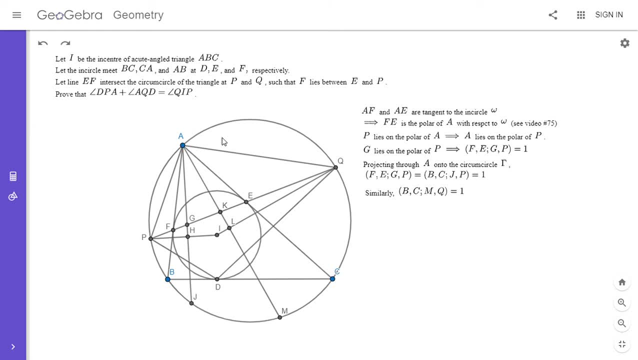 but the other two are different and they're all points that lie on the circle. then that means that J, Q and PM have to concur on BC. So I just knew this right away because I'd seen it before. But I'm going to prove it out for you, just for clarity. So how do we prove from these two cross? 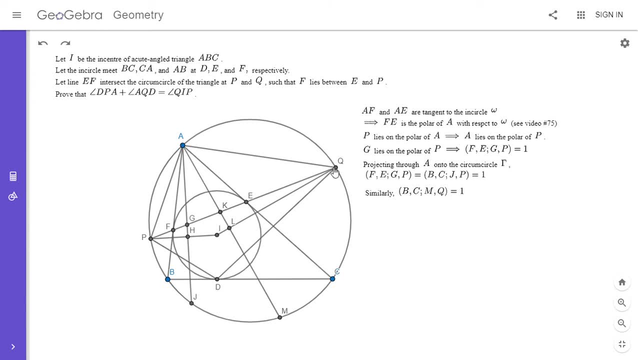 ratios that that's the case. BC, PM and J Q are concurrent. What I'm going to do is I'm going to let P- Q intersect BC at a point N. Okay, and where do I go from here? So we have the cross ratio BC. 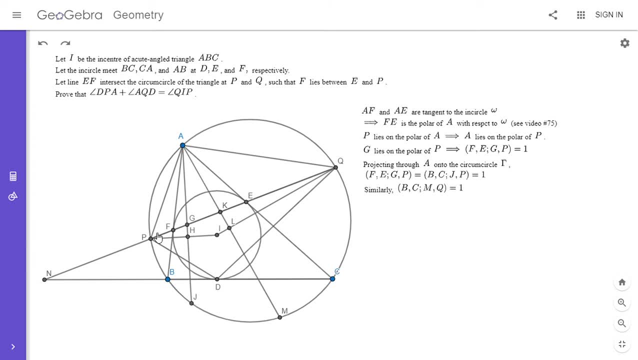 J P, and what I can do is I can project this four points through point Q. So that's what I'm going to do Now. I'm going to hide the in-circle in point D temporarily, and you'll see why later. So we need the in-circle to construct. 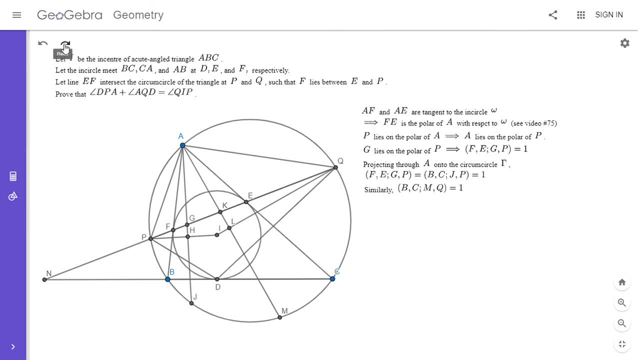 the whole problem, but I'm going to hide it for now for reasons that I'll explain soon. Okay, so I'm going to take those four points, So I'm actually going to start with BC, J and P and I'm going to project them through point Q. 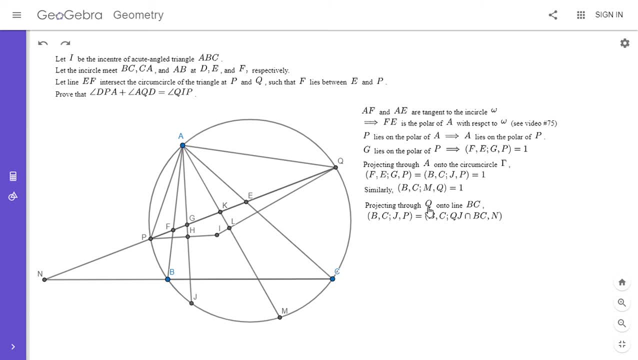 onto the line BC And I knew to do this because I'd seen it in other problems before. So B and C still stay at B and C. But if we project point P through point Q it goes to point N on the line BC. 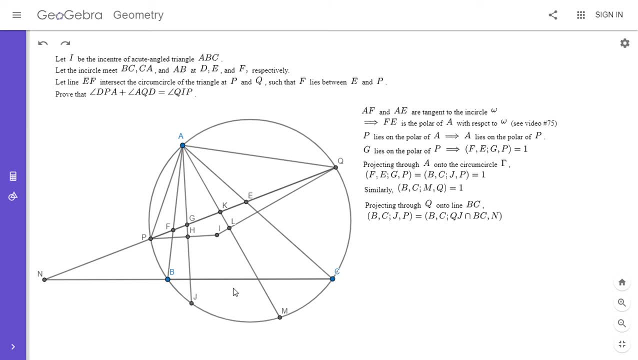 And if we project J through point Q, I'm just going to label that as Q J intersect BC. So I'm not going to draw the point Okay, and then P, Q and P, and I'm just going to label that as Q J. 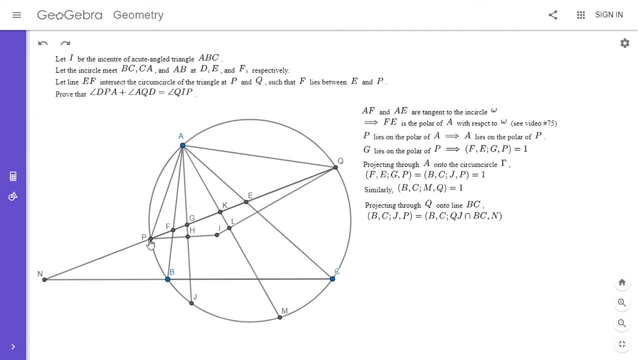 intersect BC. So I'm not going to draw the point, Okay, and then P, Q and P and I'm just going to go to point N. So we have this: cross ratio is equal to BC, and then this intersection point of 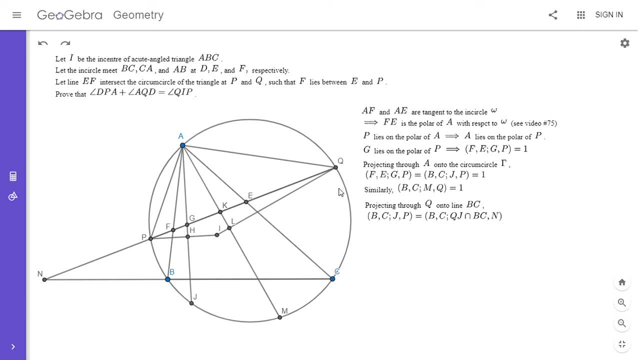 Q, J with BC, which I'm not going to draw, and point N, Okay, and then I'm going to do the same thing with this other cross ratio, but I'm going to project through point P instead. So if I start, 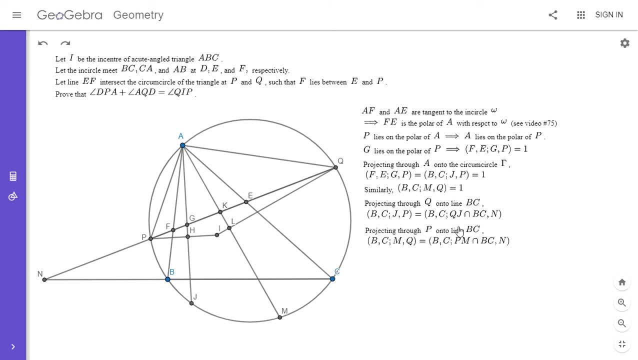 with BC, M, Q and I project through point P onto the line. BC, B and C stay where they are. If I connect P to point R, I'm going to project that as Q, J intersect B, C and then this cross ratio is equal to BC. 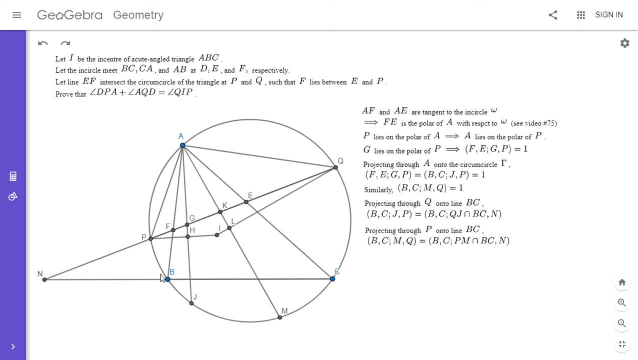 connect P to point M, it intersects BC at PM intersect BC. I'm just going to leave it like that. And if I connect P to point Q, it intersects line BC at point N. And the reason I did that is because now we can compare these two. They both have to be equal to one, But BC and N are the same. 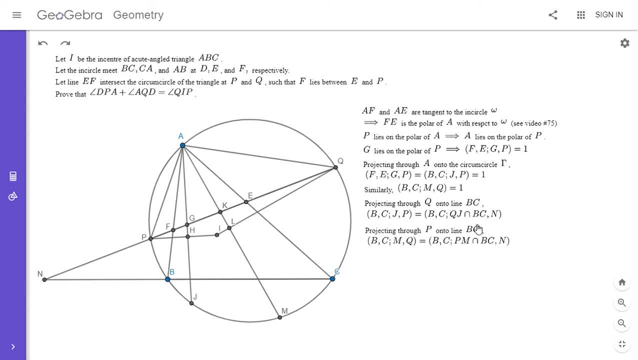 in these two cross ratios. So that means the third point, which is QJ intersect BC has to be the same as PM intersect BC. That's the only way they could both equal one. So this is a very well-known fact, but if you haven't seen it, I'd recommend trying to prove it. All right. So QJ intersect BC is the 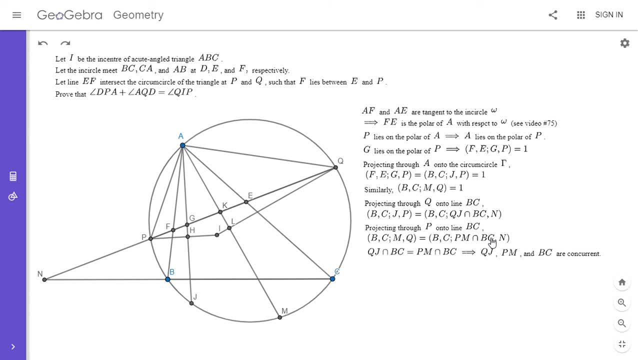 same as PM intersect BC. So what does that mean exactly? If I connect P to point Q, it intersects line BC at point N, And if I connect P to point N, it intersects line BC at point N, And if I connect P to point Q, it intersects line BC at point N. 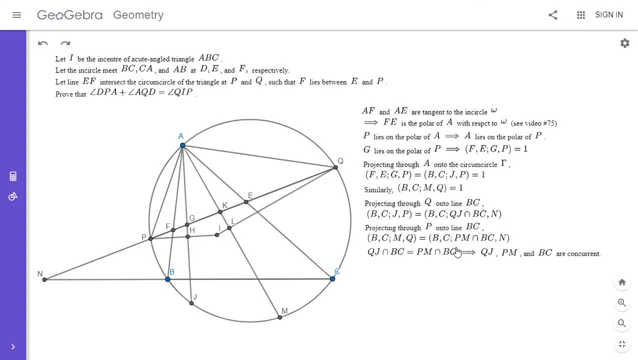 So if QJ and PM intersect BC at the same point, then they have to be concurrent. All right, So now we're really getting somewhere. So I'm going to call that point R. And if they all concur at point R, then this cross ratio BCRN has to equal one. 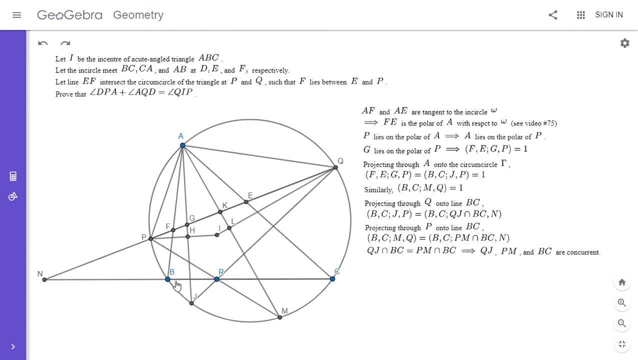 So where do we go from there? So the cross ratio BCRN is equal to one And if you watch my first video on projective geometry on my channel, if that cross ratio is one and we have EF intersecting the line BC at point N like this: 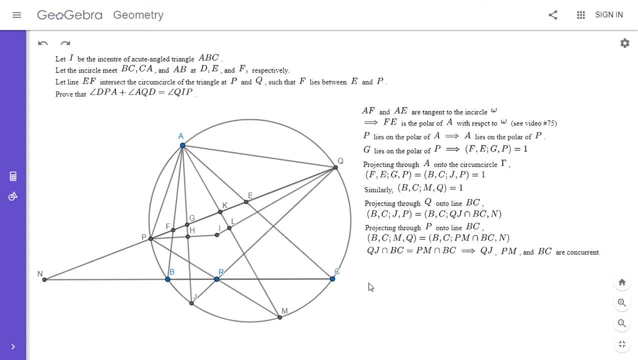 then that means that AR, BE and CF have to be concurrent. So in that video I actually proved the converse of this, but it's not easy to show that this also, I'm sorry, it's not too hard to show. So I'm going to call that point N. And if you watch my first video on 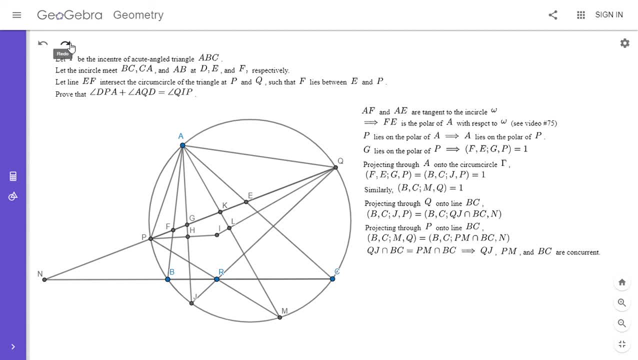 that this also has to be true. So, I'm sorry, ignore that. Okay, So since BCRN, since that cross ratio is equal to one, then BE, CF and AR have to be concurrent, But E and F. those are the points. 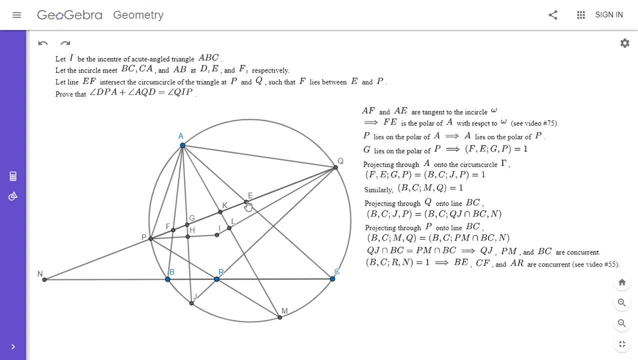 of tangency of the N circle, And so that means that R also has to be the point of tangency of the N circle, Because the lines connecting each vertex to the point of tangency of the N circle with the opposite side, those are all concurrent at the Jergaon point of the triangle. And if you don't know, 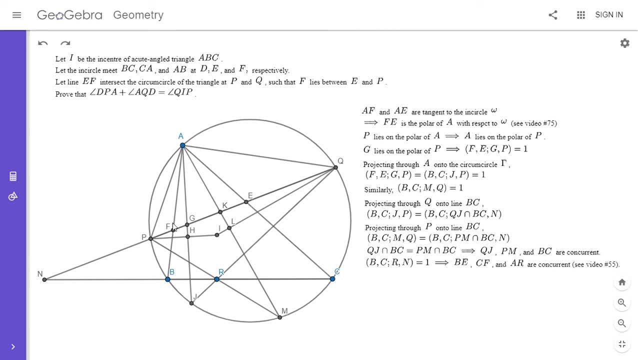 about this. it's very easy to prove by Cheva's theorem. So- and I do prove it also in another video- So R has to be the same as the original point D, which was the point of tangency of the N circle with BC. 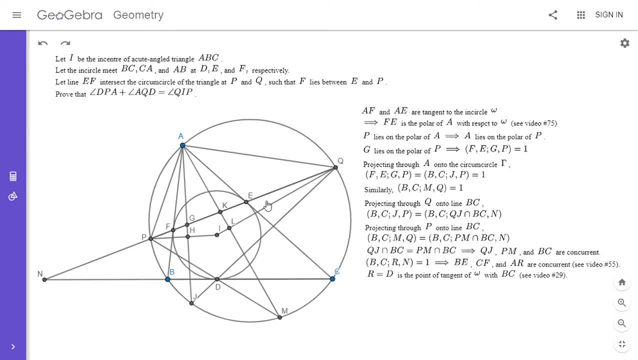 And that's because AD, BE and CF are concurrent. And if you'd like to see a proof of that in a video of mine, you can watch video number 29.. Although it's not too hard to show by Cheva's theorem, since the tangents BD and BF are equal, AF and AE are equal and CE and CD are equal. 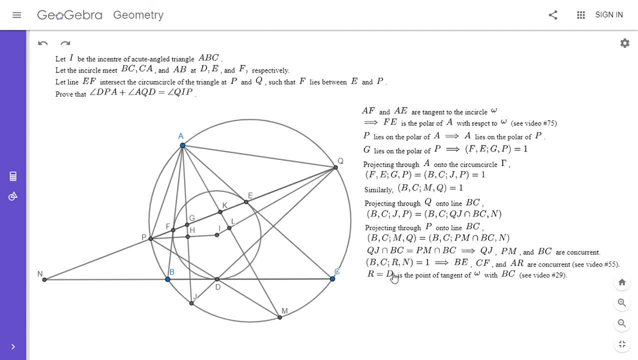 All right, So R is equal to D, And so this is really enough to conclude the problem just through angle chasing. All right, So I'm going to explain that here. Okay, So we want to show that angle QIP is equal to the sum of these two angles. 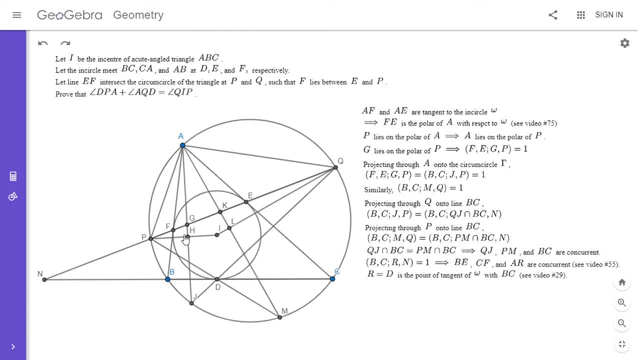 But angle QIP it's the same as angle LIH And if you look quadrilateral AHIL that has two right angles, So we can make use of that. So angle LIH has to be 180 minus angle HAL. So I'm going to write this out. 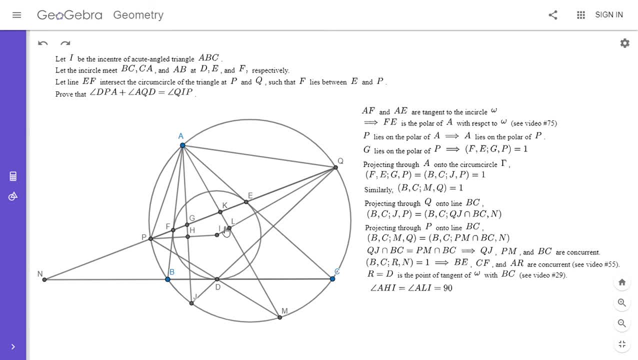 So angle AHI is equal to angle ALI, which is 90 degrees, And so that's because we constructed those two lines to be perpendicular to IP and IQ. All right, So that means that angle QIP is the same as angle LIH, which is 180, minus angle MAJ. That's because in this quadrilateral 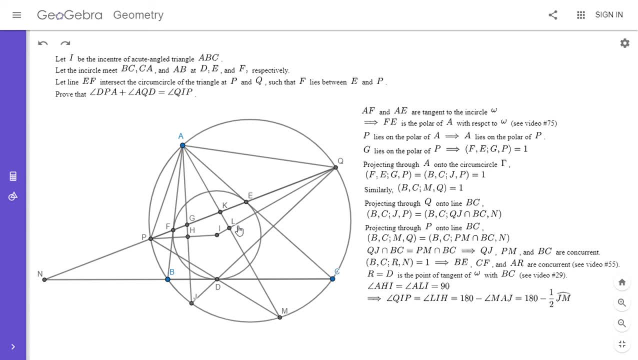 two of the angles are right angles. So since LIH is one angle, the other angle has to be 180 minus angle LIH. So LIH is 180 minus angle LAH, which is the same as 180 minus angle MAJ And angle MAJ. that's half of arc JM in the big. 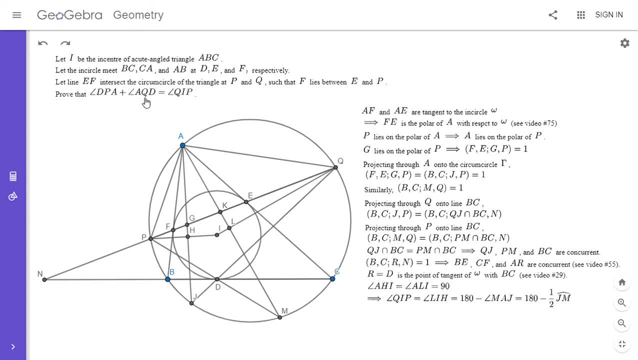 circumcircle gamma. All right, And now I'm going to do another angle chase with these two angles, So angle DPA and angle AQD, All right. So angle DPA plus angle AQD. Well, angle DPA, that's the same as angle MPA. Now that 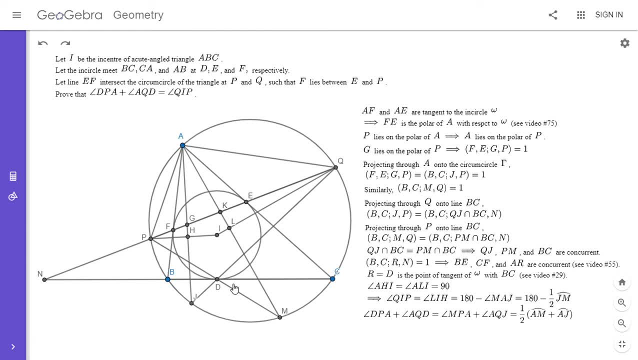 we know that that concurrency point is point D And similarly, angle AQD is the same as angle AQJ And each of those are half of their intercepted arcs. So angle MPA is half of arc AM And angle DPA is half of arc AJ. Okay, So this is half of arcs AM plus AJ, But if we try to compare these two, 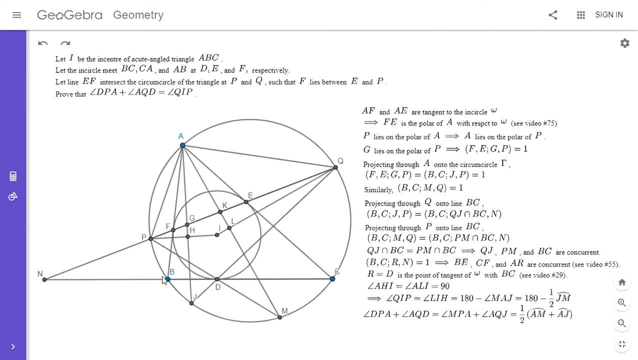 arc AM plus arc AJ is 360 minus arc JM, since those three arcs comprise the entire circle. So half of the sum of AM and AJ is actually half of 360 minus JM. That's the same as angle QIP, And so that solves the problem. So for this problem I feel like 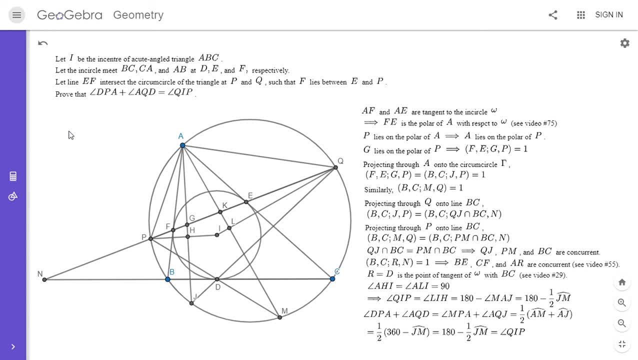 knowing about poles and polars really helped a lot with the solution. If I didn't know about poles and polars, I'm not really sure where I would have started on this And my solution. it happened to be the same solution as Evan Chen's on the forum, So I think his solution may have been the